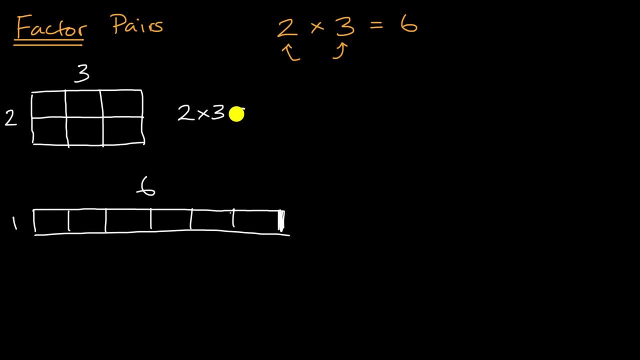 So that would be another factor pair. We know that two times three is equal to six and we know that one times six is equal to six, And these are actually the two factor pairs for six, and we can do it with larger numbers. 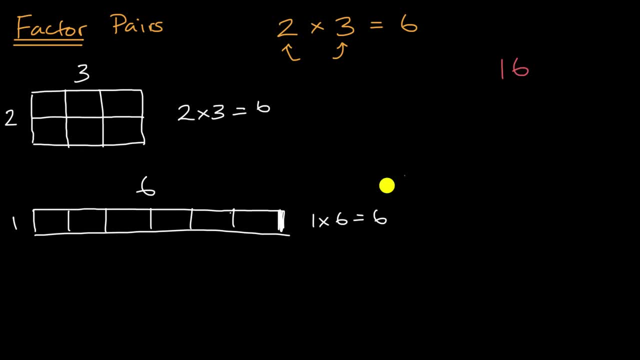 We could think about: what about all the factor pairs for something like 16?? Pause this video and see if you can figure out what that is. Pause this video and see if you can figure out what that is. Well, I'll set up a little table here to think about that. 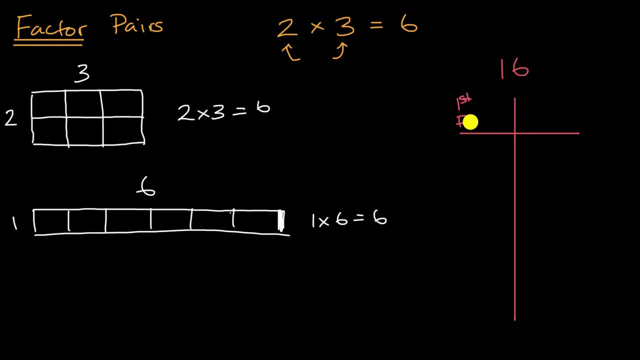 And so in this column I'll put the first factor and in this column I'll put the second factor. And the way I like to do it is I start at one and I keep working up to the number to try to figure out all of the factors. 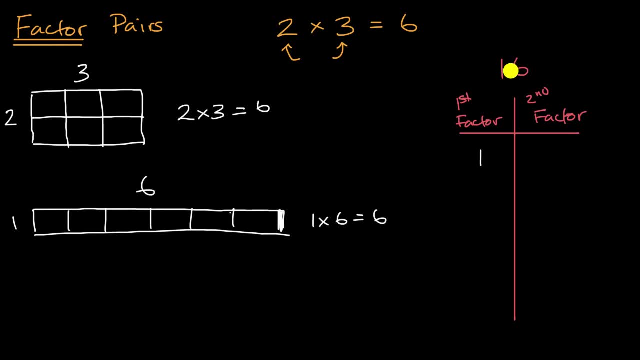 So let's start with one. So one is definitely divisible into 16, and as long as you put a whole number here, it's going to be divisible by one, and then we'll have to multiply by one to get to 16.. 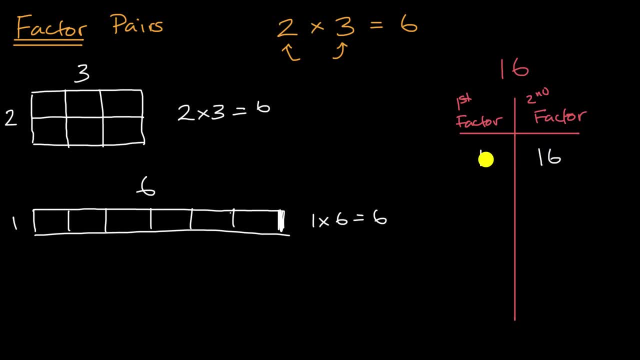 We'll have to multiply it by 16.. So that's a factor pair right there, one and 16.. Now what about two? Does two go into 16?? Well, sure, two times eight is 16, so that's another factor pair, two times eight. 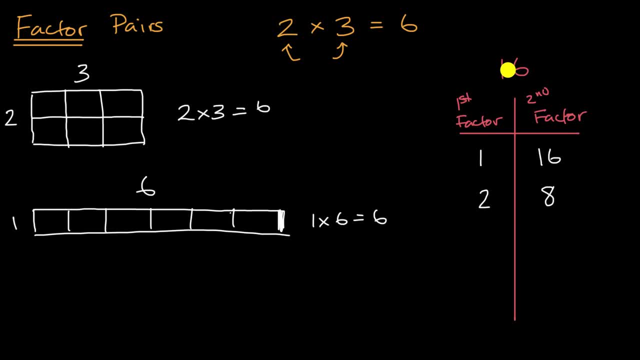 We found another factor pair. Now what about three? Does three go evenly into 16?? Well, no, three times five is 15, and three times six is 18,. so three doesn't go into 16,. so three would not be a factor of 16.. 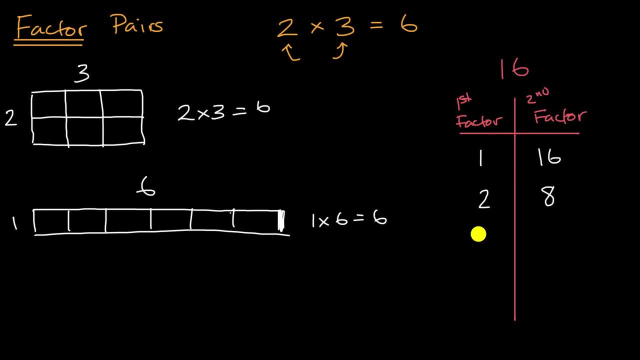 What about four? Well, four times four is 16, so that's a factor. pair there, four and four. What about five? Well, no, five times two is 10,. five times three is 15,, five times four is 20.. 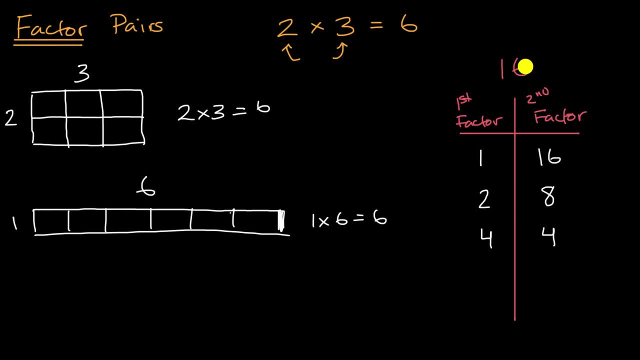 Five does not go evenly into 16.. Same thing for six. six times two is 12,. six times three is 18, does not go evenly into 16.. What about seven? Seven does not evenly go into 16.. Seven times two is 14,. seven times three is 21.. 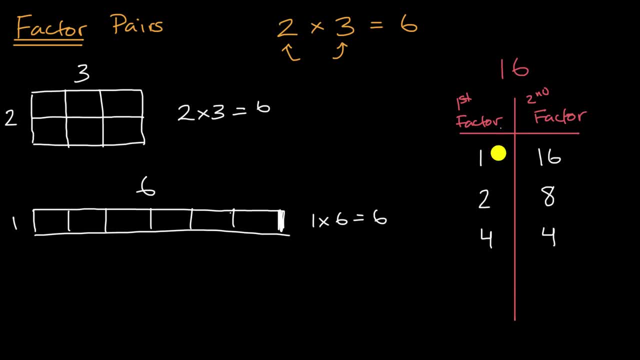 What about eight? Well, we already know that eight goes evenly into 16.. You might be tempted to say, oh, there's another factor, pair of eight times two. but we already wrote that down. We just happened to say that two is the first factor.